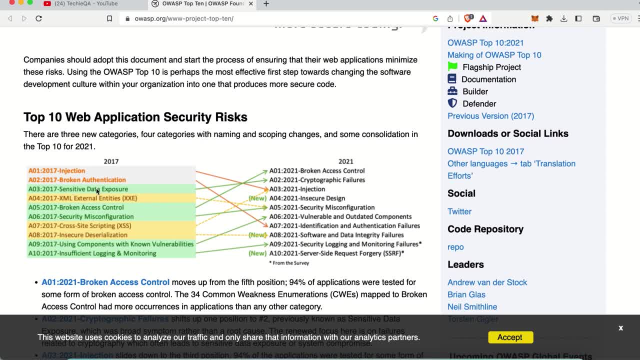 sensitive data to the public or like to everyone, is a problem. so XML, external entities, so broken access control, like everything, cross-site scripting, JavaScript injection- we can do using comfort, known vulnerability, insufficient logging and monitoring. so everything is like one or the other way it's useful to. 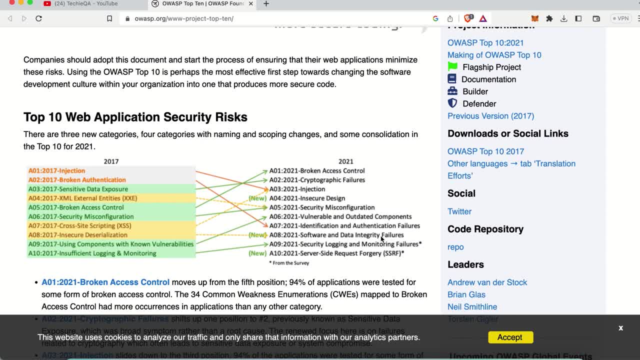 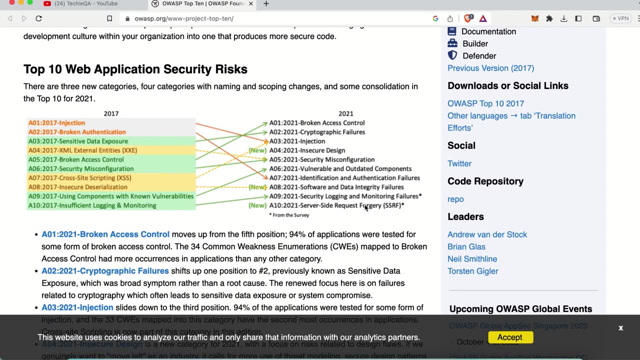 fix the issue. so there are, for example, in swing logging and monitoring and all will come under low priority. but broken access or across its scripting, injection, D stuff and all will be like a priority to high level. so based on the stuff it will be prioritized. so whatever the application, 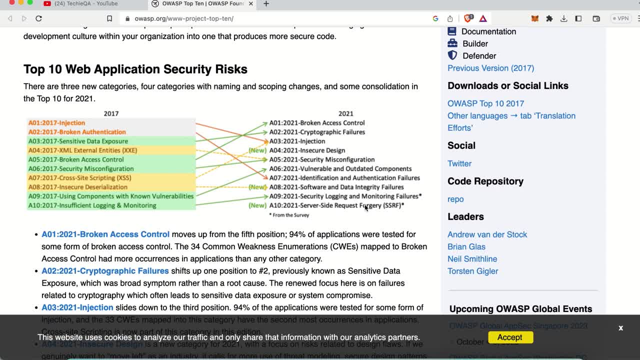 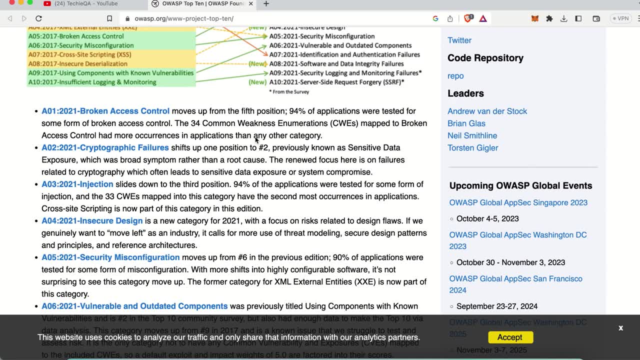 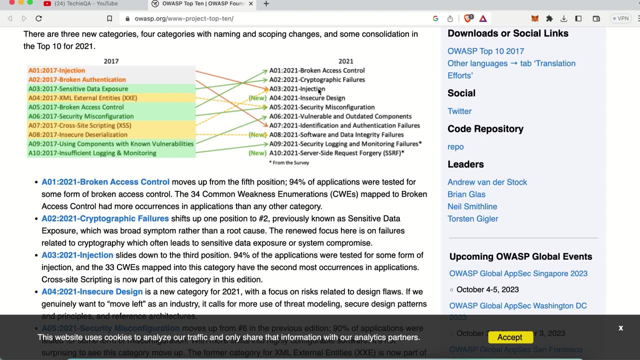 we are going to test. so the, the tool will automatically test, like all this top 10 one. so but once you get the report rate, if you want to understand what is that report means, like before that, you have to understand this stopped end standards. what is the actual issues? okay, so just. 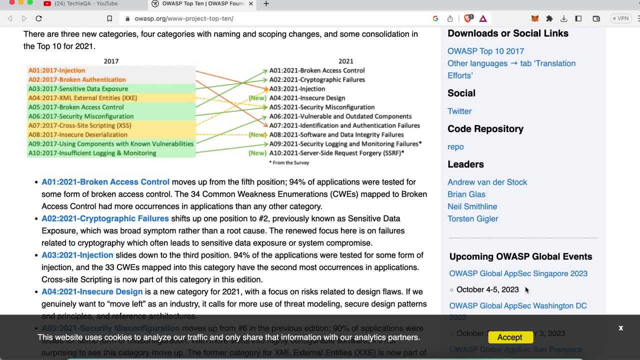 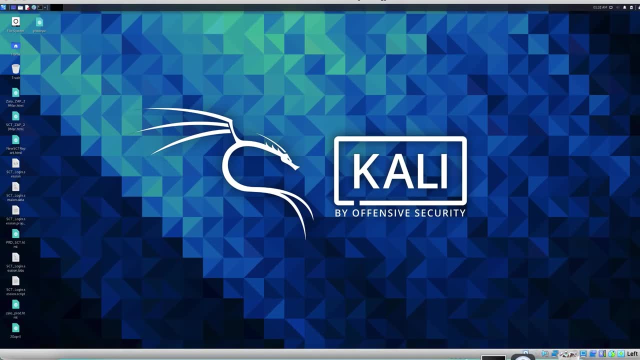 about it, then it will be easy for you. also, I'm going to use Kali Linux for this, because Kali Linux is like kind of security offensive security test OS which is like it's almost like similar to Linux, but it has lot of tools, like available for testing the security. so 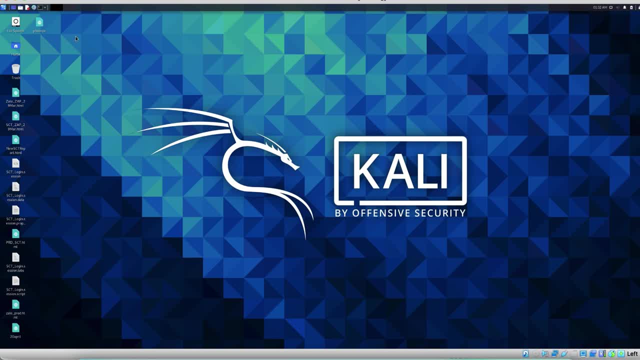 in this tutorial we are going to use Zap, OASP, Zap, like once you are going to here you can see web application analysis, Zap. so actually I'm using virtual box, kind of a VMware. I have installed Kali Linux on this and I'm using it okay. so if you have a separate system, you 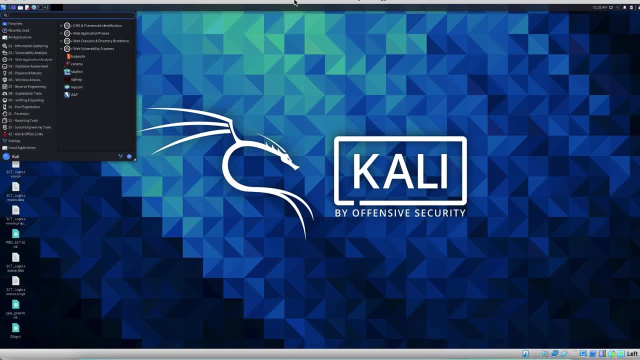 can install Kali Linux or you can use VMware. So let's see how it works. Also, Zap is available for the Windows Mac standalone version also you can download, but it's not like looks good for me, so I taken the Kali Linux only so you, if you have the 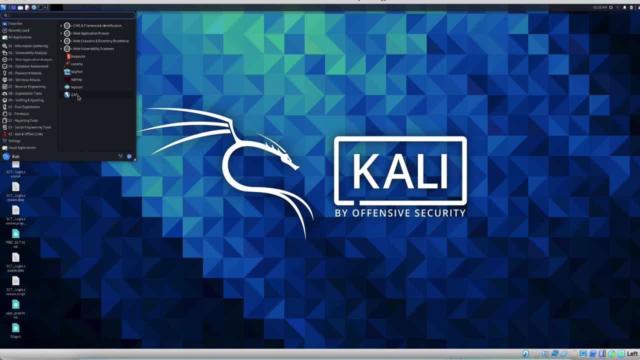 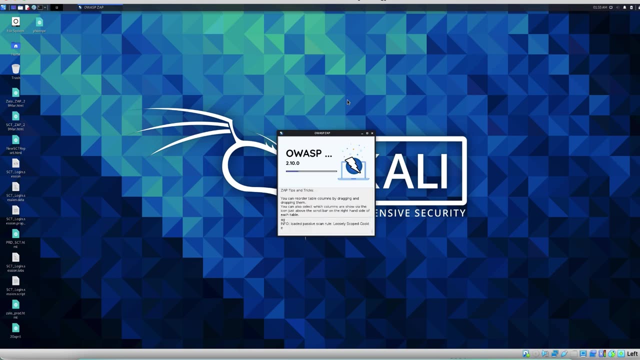 system. just install the Zap Community Edition or free version. just try it out in your system. only okay. so I'll just open Zap. also, we need some sample site. let's see. I'll take a techy QA site maybe, so once it open it's. I'm using 2.10 which is in build with. 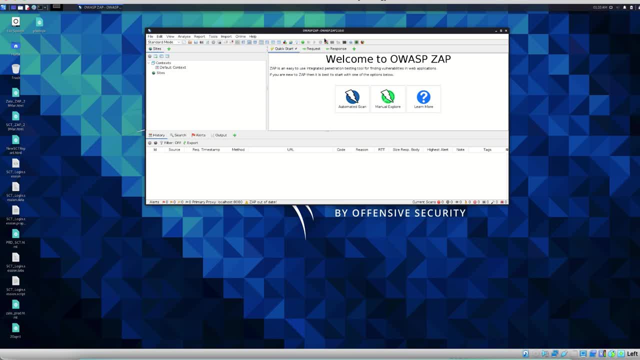 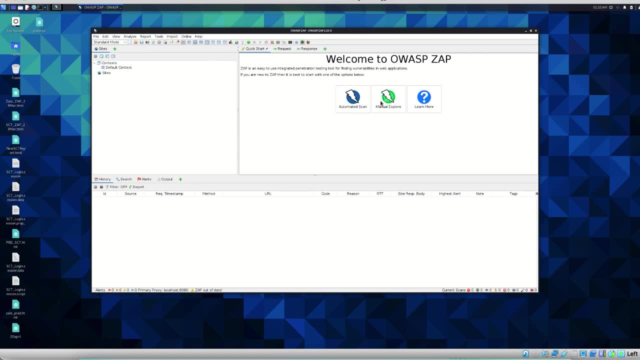 the Kali Linux. you can use the latest version. so here is the UI. UI will be look like this. so there is two of like three option. two option actually is help site automated and manual explore. so automated what it will do that site. it will automatically download the site. 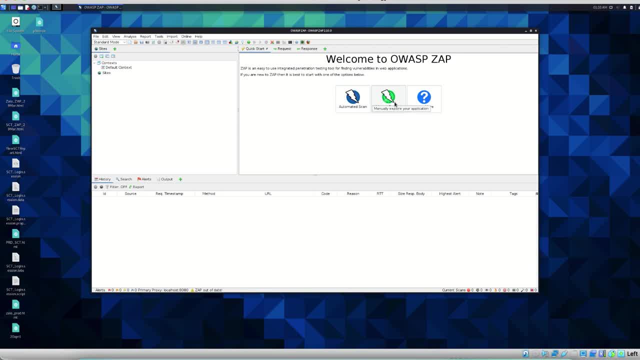 that is, auto modernize, not just be a subscription into commentaires and all allowing you to do all the action. and try to find the URL and do it manual. what it is like? it will open the browser you have to explore yourself. so manual one we can see other day and automate. 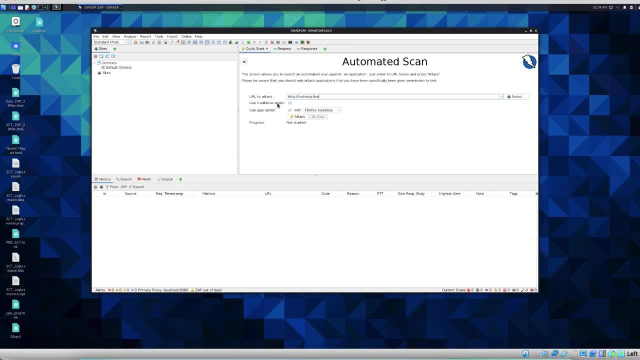 1. we can start doing it, so maybe what I'll do, the Light It's just a way. a small web page, it doesn't have much links or backlinks and all there, So use traditional spyro. Just check on it. 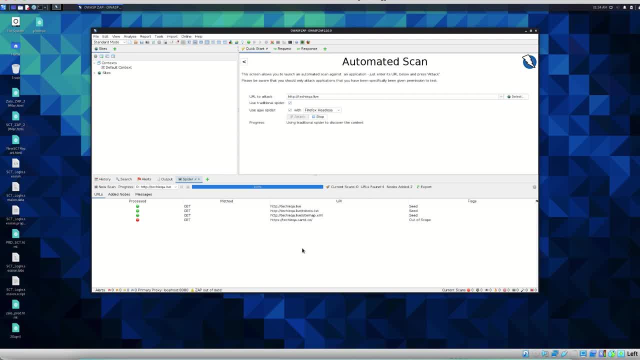 Firefox just start attack. so once you start attack, you can see all the urls here. it will just try to get all the url and try to find all the vulnerabilities in the website. let's wait for the report. yeah, now we can see how many requests sent here. 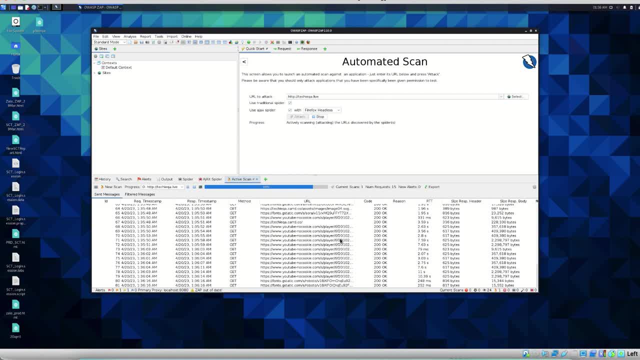 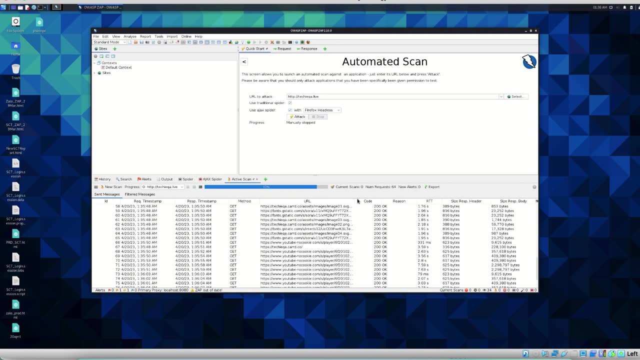 so it will check links, whatever associated with this site. uh, so once all the check is done, it will just end and it will show the report. so what i'll do for the tutorial? i'll just stop it manually. uh, we can see the report how it look like. we can see all the request and all sent here. so current scan is zero. so it stopped. 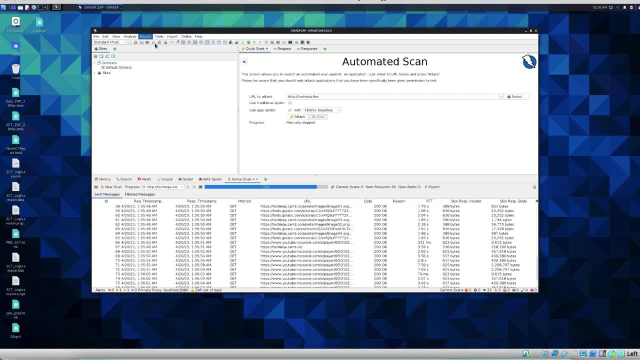 currently. so you, you can you just directly go to report and generate html. so it will generate html and it will open with the browser. so maybe, uh, i'll just save as a file. so once you saved, it will be open with the browser. inbuilt browser, whatever it is. yeah, uh, in this report we can see: 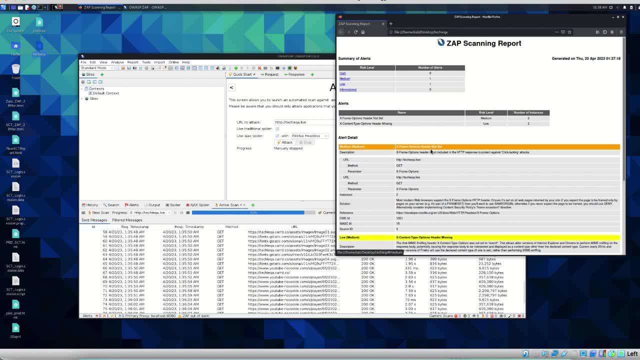 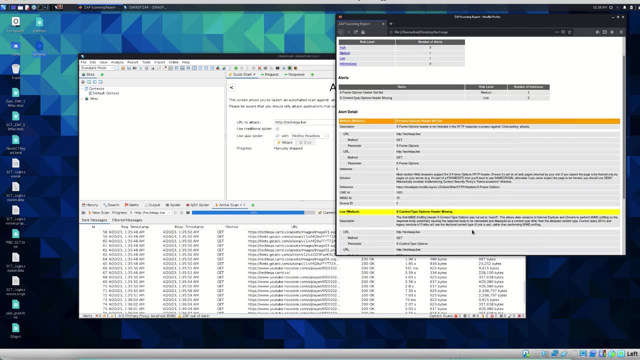 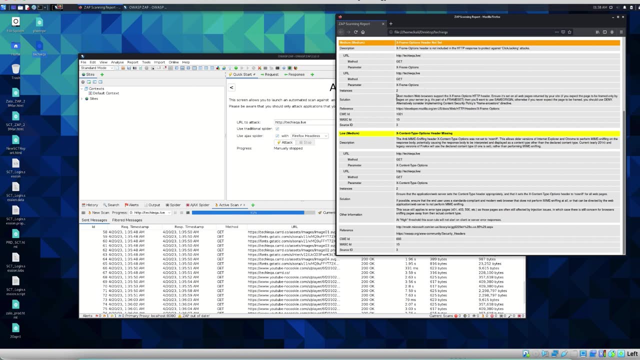 medium is one and low is one, which is related to x frame option, header not set, and one more is header is missing, which is low one. uh, it's, it's all under, like this, oasp standards, like the checks. okay, it will uh give you the url as well as uh it will give the solution most. 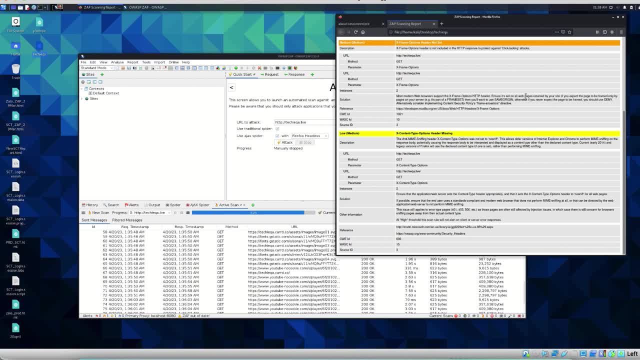 modern web browsers support x frame http. ensure it is set for all the web pages written by your site. okay. alternatively, consider implementing content security policy frame ancestors you. if you do it, it will be more secure. so it will give you the suggestion also what we have to do it okay. so if you select for other site, maybe your, uh, the site you are. 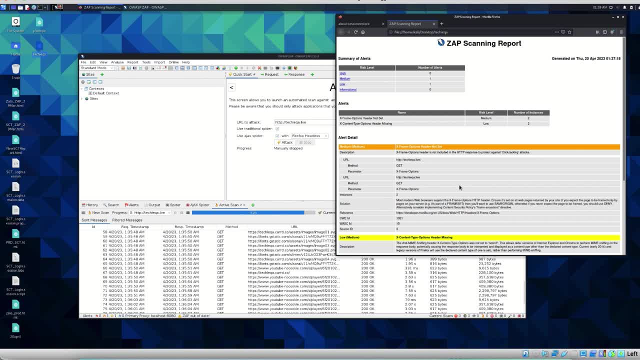 testing. so i'm i'm not able to use other site because i'm just showing your demo. even i cannot take a public site right, so it will block. uh, maybe block block my ip if i'm doing something related to security without their permissions, so don't do that. also, i'm. 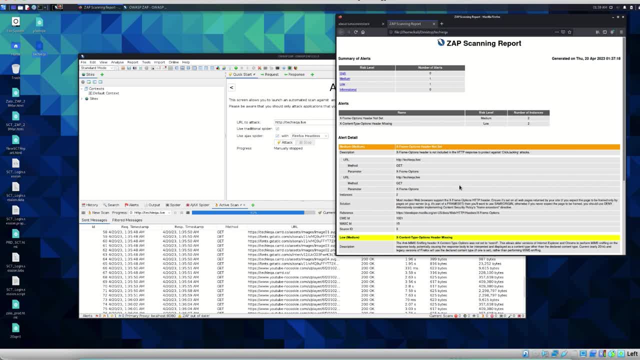 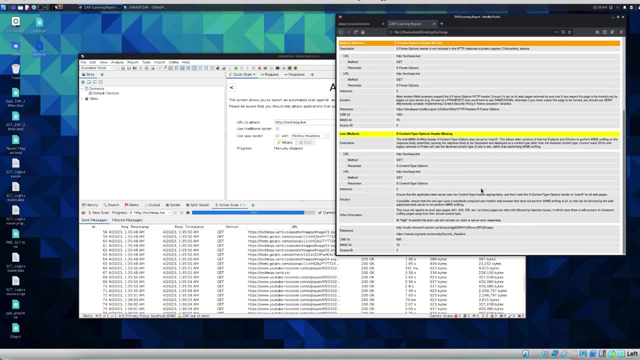 suggesting, like, whatever you are using the site, like you are testing one so that one, you have to use it. okay, guys, so uh use like uh kind of uh the site, uh, which is like having lot of links, lot of uh models. this, this side, is very smaller one. that's why you're able to see very less. 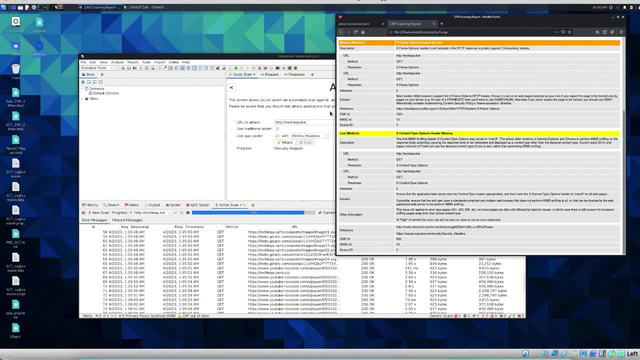 okay, okay, guys, thanks for watching this video. maybe next video i can show you how to do the manual explore, uh that also, because this one is like kind of it's automatically going to few pages and getting all the links, but uh, in the manual maybe you can, you can uh, explore the flow. 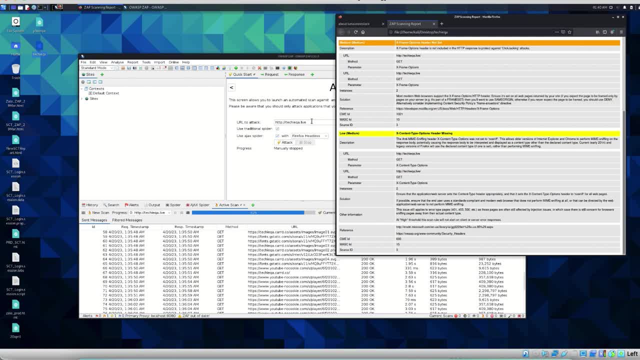 for example, amazon, if you are testing so you can check the order flow and see the security analysis. okay, so maybe in the next video you can see it. thank you guys. thanks for watching my video. if you like it, please share with your friends and subscribe. thank you.